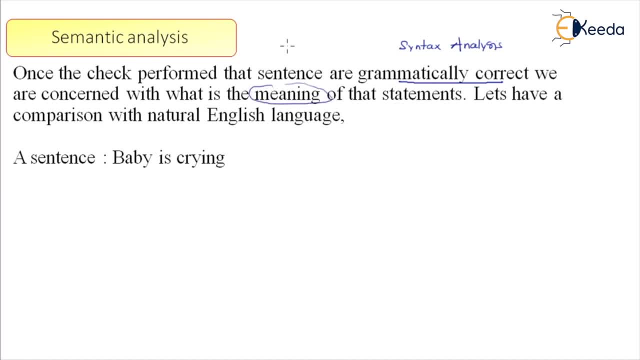 so the meaning of the sentence is: we are concerned with the meaning of the sentence. This is the important term when you talk about Semantic Analysis. We are more interested in meaning. What does it imply? Okay, so there are two parts of it. One is the static entity and 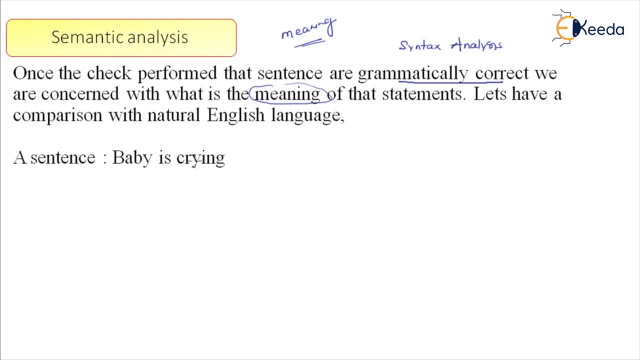 another one is the meaning associated with it. Let's have a sentence which is a very natural language, natural, which is, which is a natural language. We use this sentence in natural language. The baby is crying. Okay, now baby is crying. So what we have done is we have. first, we have 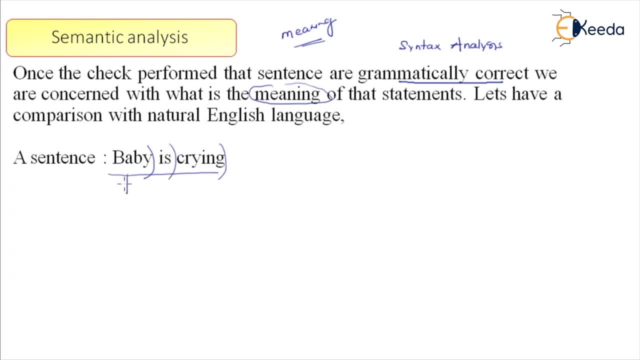 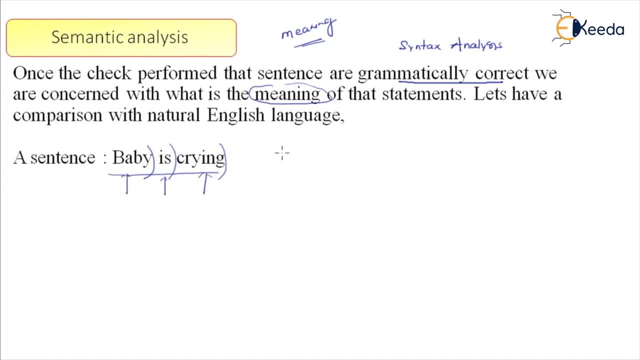 Then we have performed. whether this sentence is correct or not, okay, whether without, without, it is being syntactically correct. There is no point of analyzing the sentence Further. it has to be syntactically correct. And now what we are going to do here is is we are. 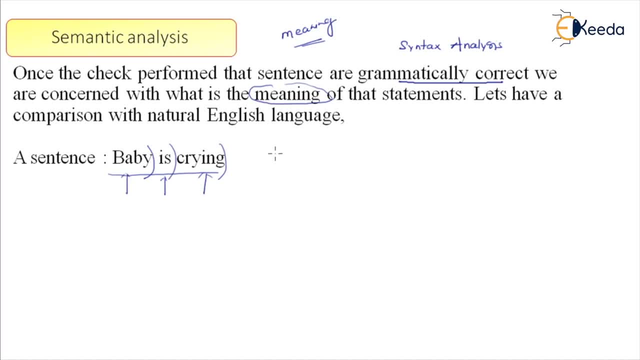 going to figure it out. what is the meaning associated with it? So when I say baby is crying, you develop a picture. let's say in your mind that there is a, there is a small baby and she is crying. So that is that we want to figure it out And for that, what we need to do here in this case. 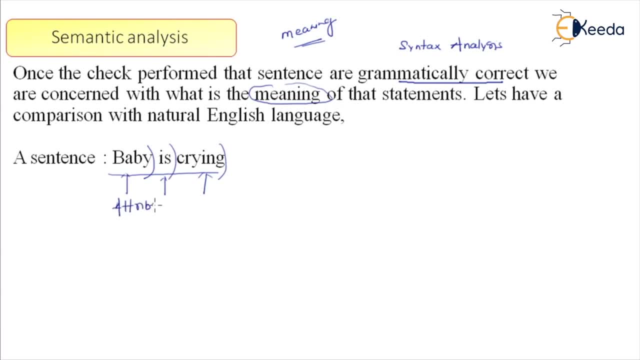 we have to associate attribute value. Okay, so each object is having its attribute value. So what the idea here in this case is, baby will have some attribute value, like the we can have, we can say edge, we can, we can say gender. Okay, so we will first describe each object with its attribute. This is a natural. 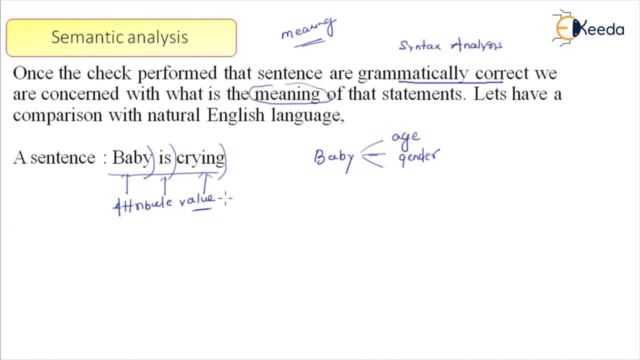 language example. And now we will figure it out by using this attribute. we will do the translation. Okay, we do the perform the translation. that what is the meaning? that the small baby and she is crying. And there can be many reason why she is crying, But we will try to develop in semantic. 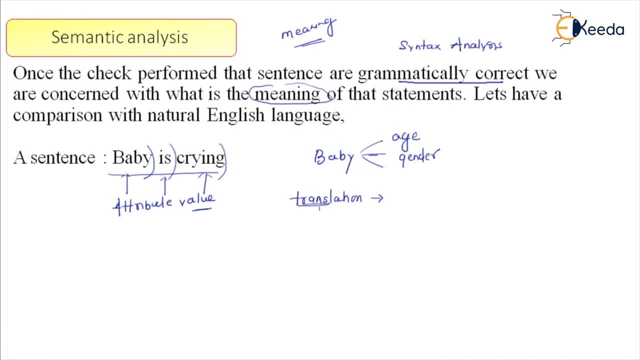 analysis, a translation. okay, we will translate the meaning of the baby and she is crying, So we will translate this thing. So this is one example. Another example can be here, like five plus six. Okay now if, if I write a grammar, let's say expression grammar and I'll say expr derive. 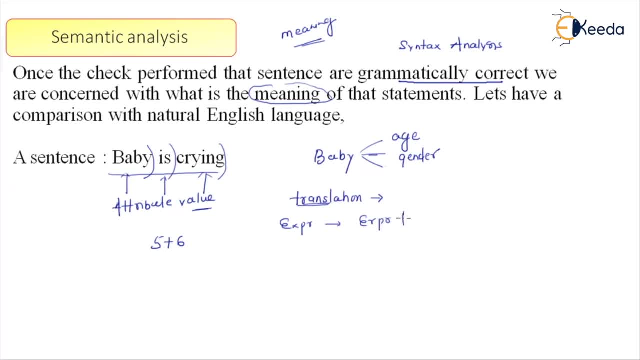 expr plus ID or ID. Okay, so now here, if I say that there is a sentence five plus six, I will say five plus six. then it will look like expression will derive expr plus ID and ID And let's say ID. 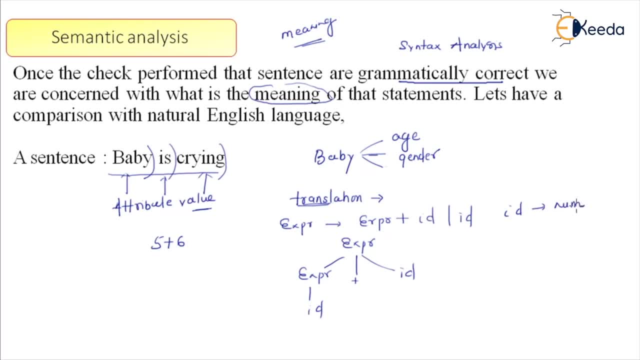 derives here a number, So this is five and then this is six. So what is this phase syntax analysis does is it will say only that five plus six. can I derive by using this grammar? Now, if I give you, without any knowledge, five plus six and I will say five plus six, can I derive by using this? 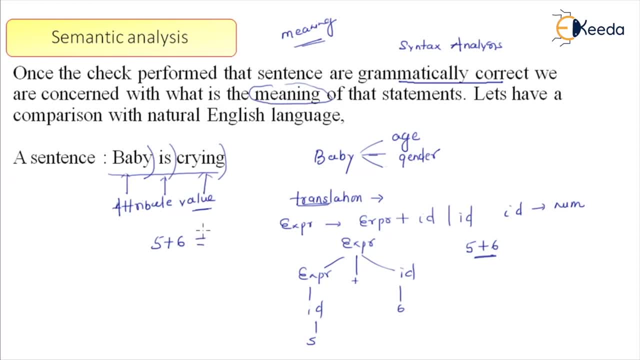 grammar. Now, if I give you, without any knowledge, five plus six and I will say five plus six and I will say, just do the translation. So what is the translation associated with it? the translation associated: five plus six. I know this is the addition operation. this is a numeric value of 56- is. 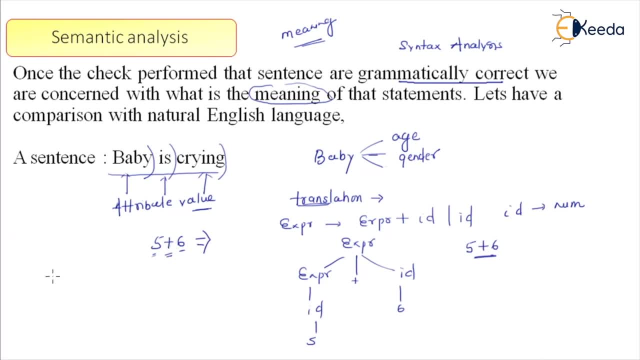 a numeric value and I have to perform the addition. So five and six are numeric value And plus means is arithmetic addition, arithmetic addition. So this comes in your mind, Okay. so look at the difference between these two phases, that one phase, 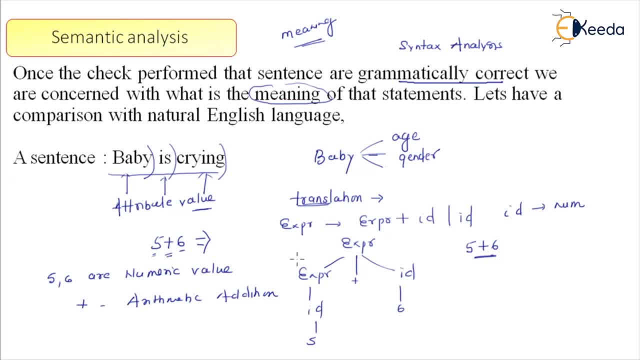 says that only five plus six is a correct sentence or not. Suppose, five in arithmetic five. if I say plus plus six, it's a trick like a mathematical statement: five plus plus six. Now, this is not a syntactically correct. I cannot translate this thing into any anything in mathematics, But when 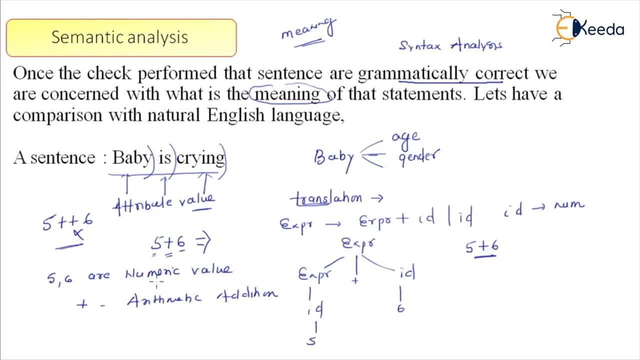 you say five plus six, immediately comes in your mind that five, six are numeric value pluses and operation, and five plus six, in context of mathematics, you can directly translate into 11.. Okay, so that sort of translation we are talking about. and this is done, finding out, figuring it. 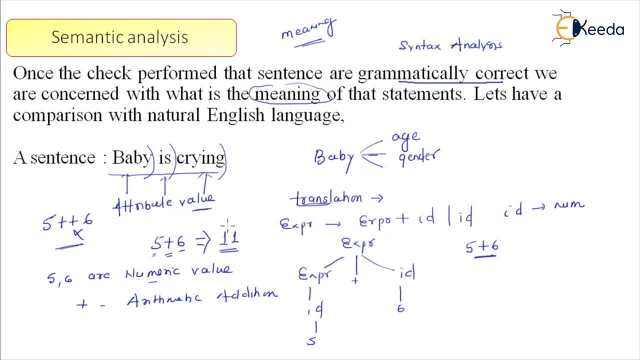 out meaning associated with the sentence is done in the phase that is called semantic analysis phase. So this phase- a few terms that you will notice here in this case- is the attribute. Attribute is the one sentence And the second sentence here is the most important. 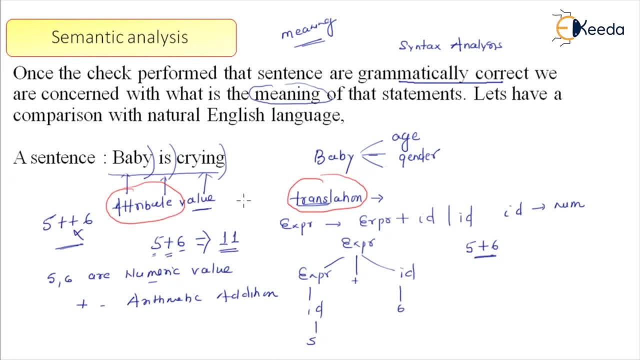 sentence is the translation part. This is still the. we are in the analysis phase And there are two most important term in semantic analysis: attribute and translation.